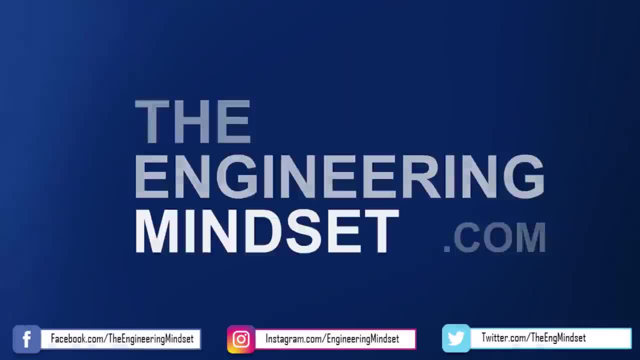 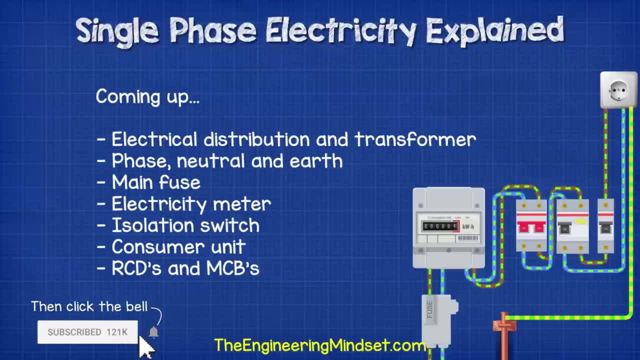 Hey there guys, Paul here from TheEngineeringMindsetcom. In this video we're going to be looking at a typical single-phase electricity supplier into a domestic property. We're going to look at the distribution cables and transformer, the phase neutral and earth, the main fuse. 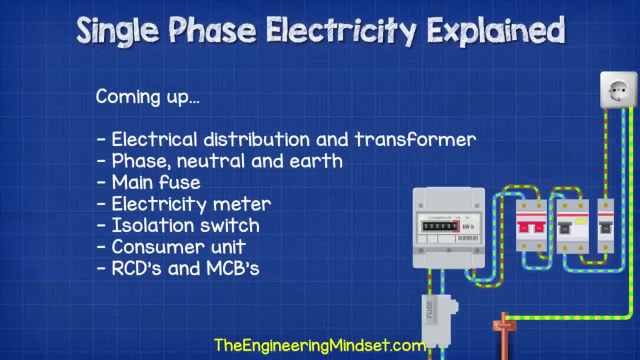 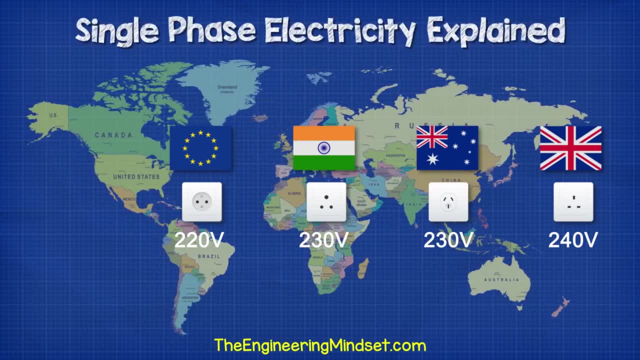 the electricity meter, the isolation switch, the consumer unit, as well as the RCDs and MCBs. Now, this is a common design used across the UK, Europe, India, Australia, New Zealand, etc. There are some slight variations and these components may look a little different between the countries. 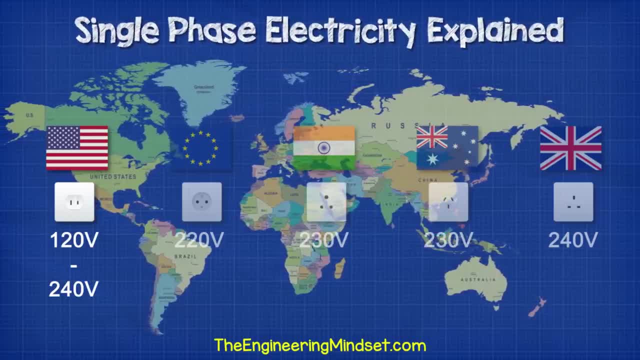 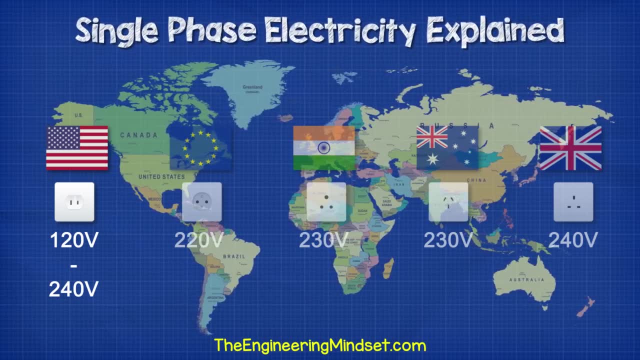 but essentially it's very similar. However, North America is a little different because they use two voltages in the homes, so we're going to look at that in detail in a separate video. You can still follow along in this video to understand the basics, though I'm going to be using the 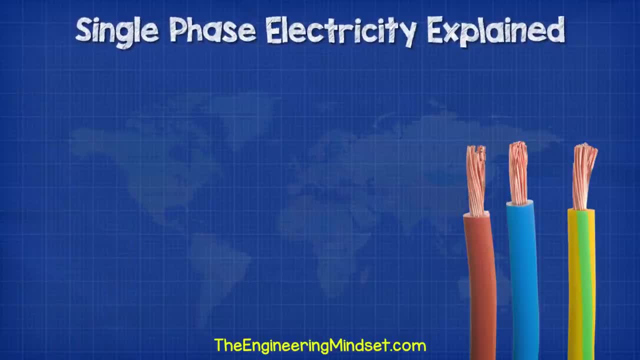 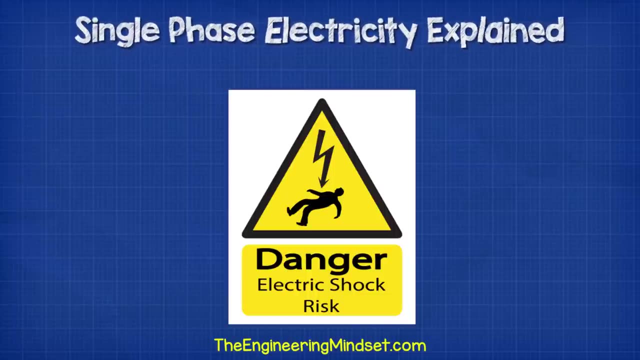 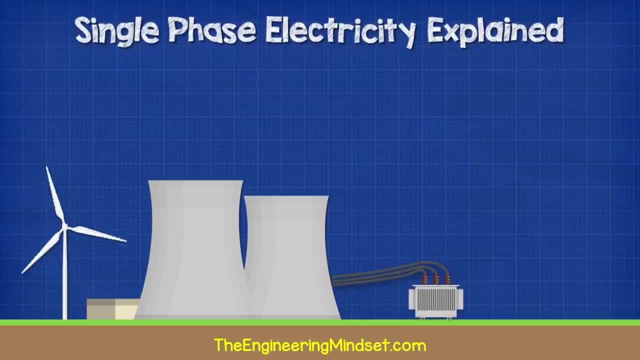 European color codes for this video that may be different from your local regulations. remember electricity is dangerous and can be fatal. You should be qualified and competent to carry out any electrical work. So the electricity is generated, far away the power station, The electricity leaves the power station and the voltage is increased in a 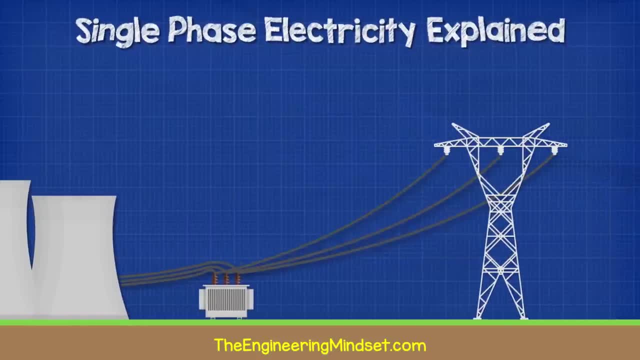 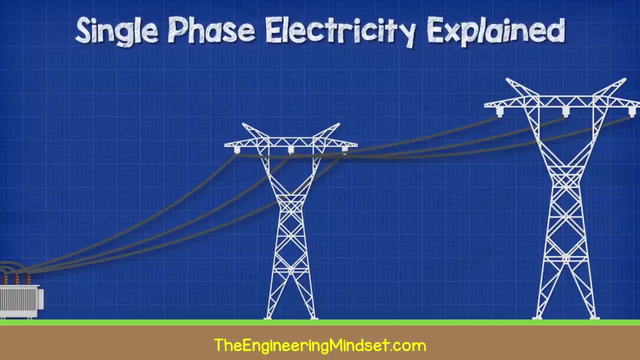 step-up transformer where it will then be distributed over long-distance transmission lines. We generate and distribute AC alternating current because it is more efficient and convenient than DC direct current. Once it reaches the town, the voltage will be reduced in a substation which is a source of energy. The voltage is then shining and listening to the current throughout. 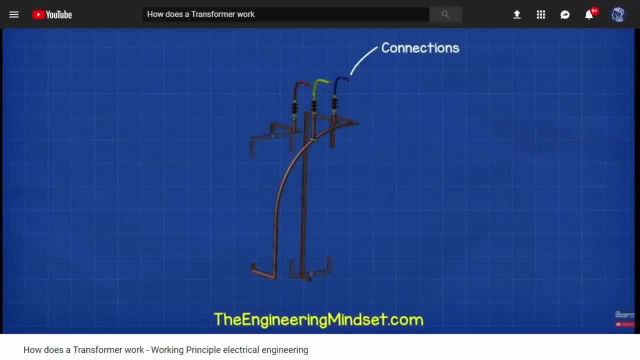 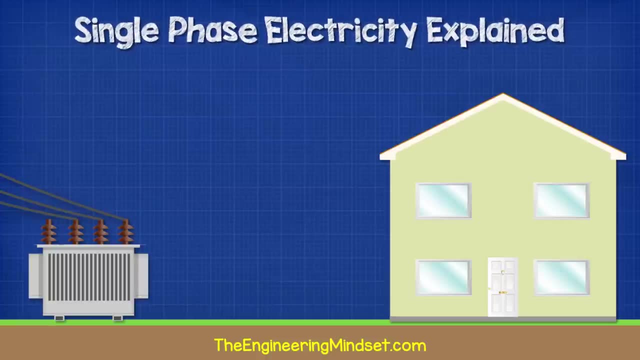 step-down transformer. If you want to learn how transformers work, we've covered this in a previous video. do check that out. links in the video description below. From the substation, the electricity will either be distributed locally through overhead or underground cables. 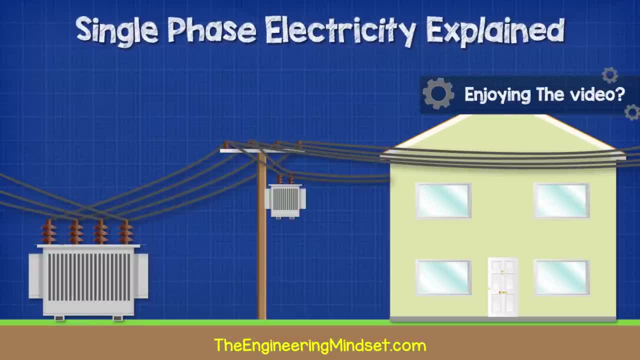 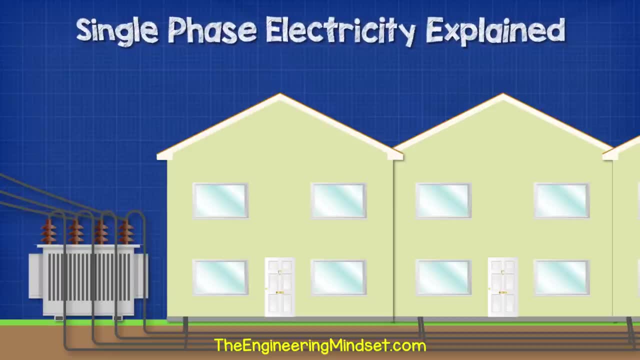 Depending on the local design and the voltages being used, a home might be connected directly to a small transformer located close to the property, Or, alternatively, a group of houses will share a larger transformer. The electricity is distributed in three phases, but in this case we're looking at 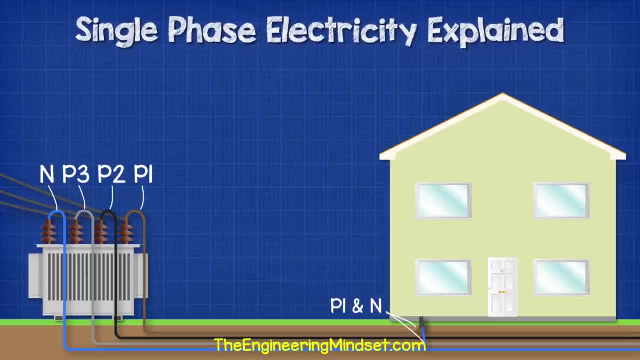 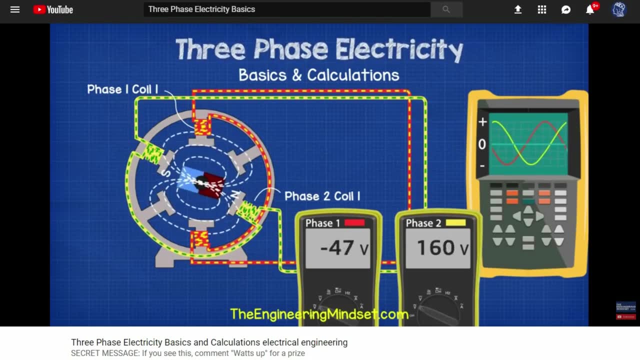 a single-phase installation, which means the property is connected to just one of these three phases as well as the neutral. We've also covered how three-phase electricity works in a previous video. do check that out. links in the video description below. 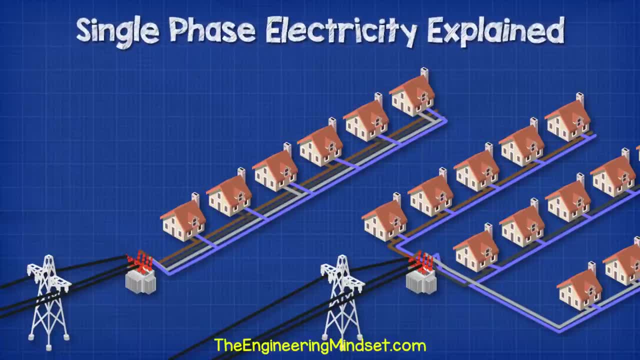 Now each house in a street might be alternately connected to a different phase, or different streets might be connected to different phases. This is just to try and balance the demand on the transformer. A smaller service cable comes off the distribution cable and will feed the property. 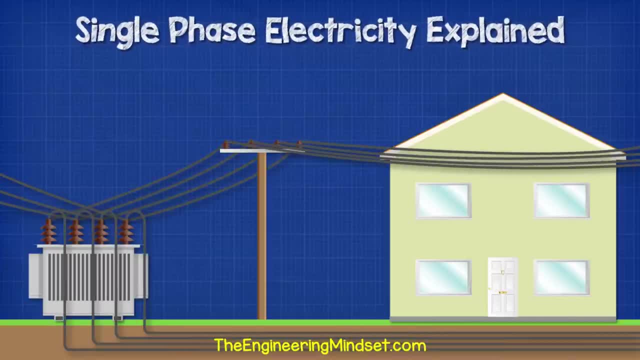 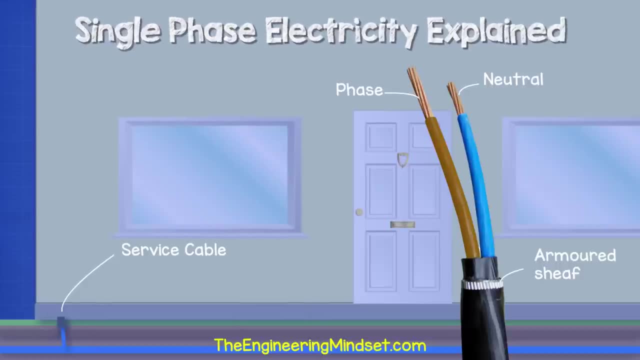 This service cable will again be overhead or underground, depending on the local installation. The service cable contains the phase and neutral wires. There's also a metal protective sheath around the cable. in most cases, especially if it's buried underground, The service cable comes in. the electricity is going. 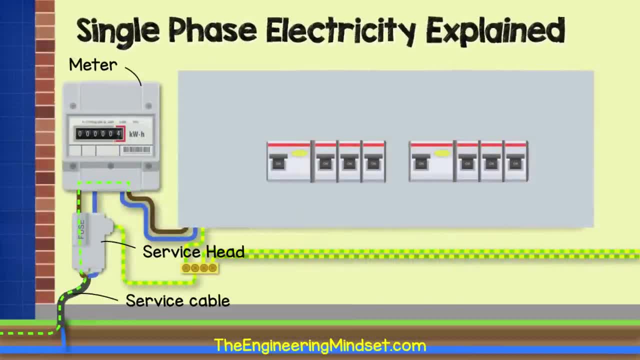 to flow through the phase pass: through the main fuse, then through the electricity meter and then into the consumer unit. The service head or cutout holds the main fuse or service fuse. This fuse provides protection to the property and ensures only a set amount of current. 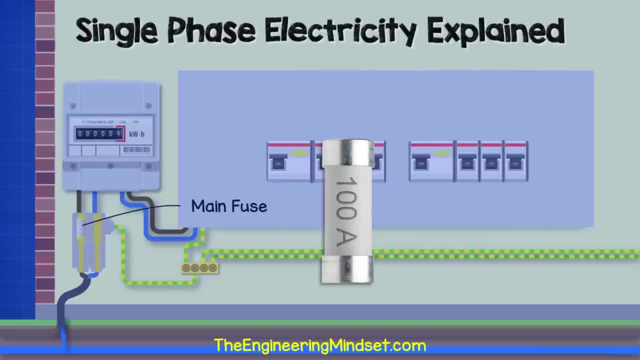 can flow into the property. For example, in the UK it's typical to have a fuse rated between 60 and 100 amps. The electricity distribution company may also remove this fuse to isolate the property. They may do this, for example. 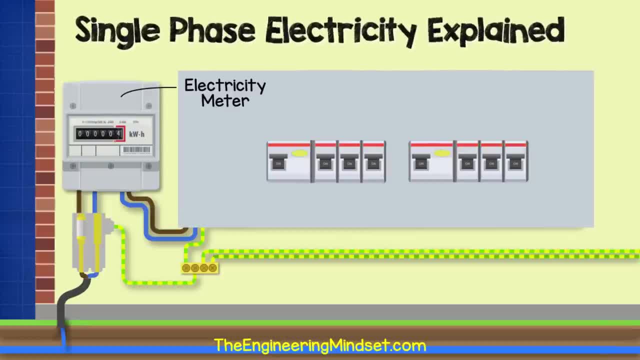 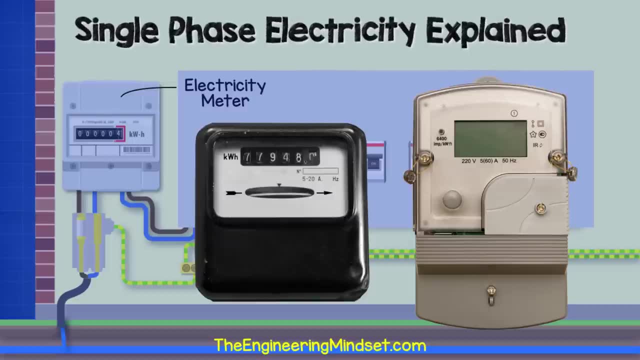 to replace the electricity meter, The phase and the neutral, then enter the electricity meter which quantifies how much energy is being consumed. We find that this meter is mechanical or electrical, or even a digital smart meter. There are a lot of variations of design for these. 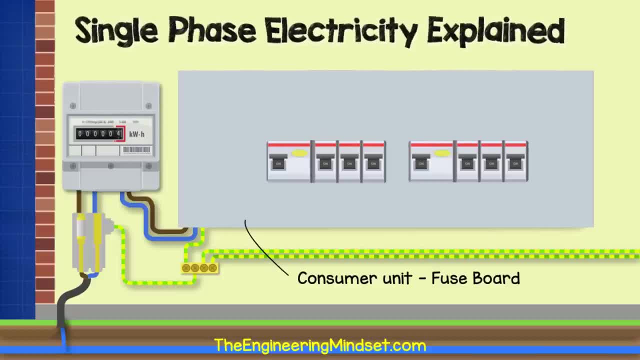 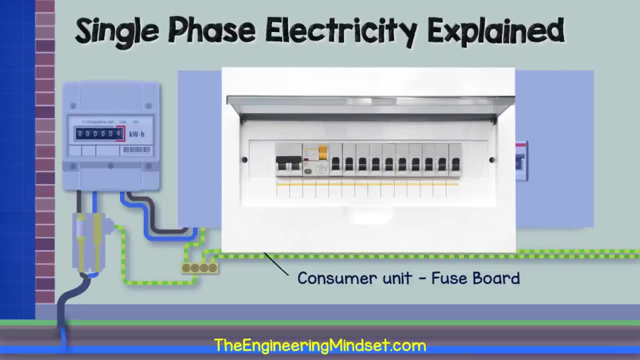 The phase and the neutral will then leave the electricity meter and enter the consumer unit or fuse board. The consumer unit or fuse board varies in size depending on the size of the property and how many circuits there are being controlled Inside the consumer unit. we first have the main switch. 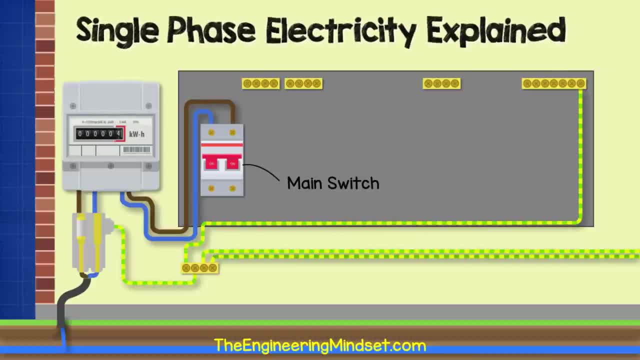 or main double pole isolation switch. This controls the supply of electricity to the rest of the consumer unit and therefore all the circuits feeding the property. This switch is not automatic and must be manually flipped to cut the power. This switch will disconnect both the phase. 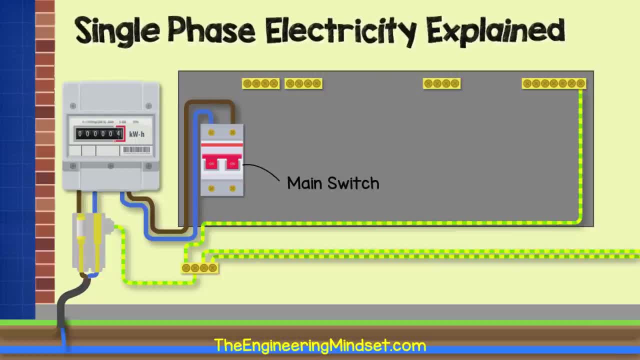 and the neutral line together. The cables typically enter the main switch via the top terminals. At the bottom we find the neutral wire which will connect to the neutral block connection. We might find one or more phase wires coming out of the bottom of the main switch to feed the RCDs. 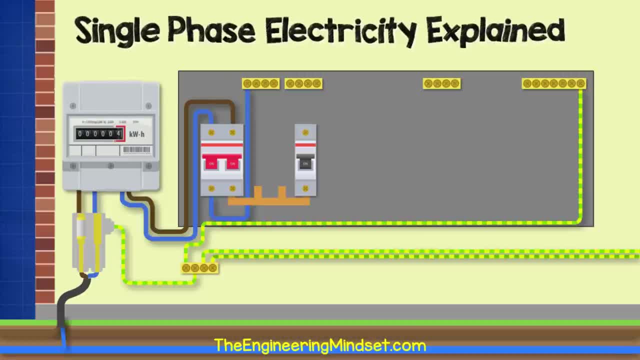 If there aren't RCDs being used, then a bus bar will feed the circuit breakers, but we'll look at that again shortly. The phase line enters the RCD or residual current device, again usually entering via the top. 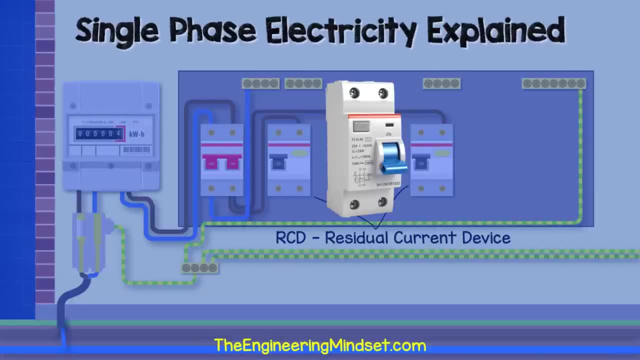 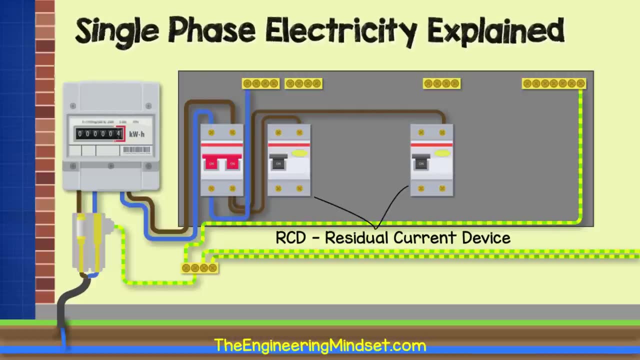 This RCD switch is constantly monitoring the electrical current. It's checking if the current in the phase line is equal to the current in the neutral line. If these two currents are not equal, then there is an electrical fault and the device will quickly and automatically. 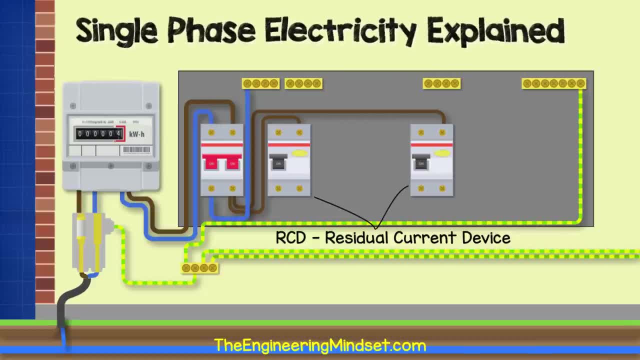 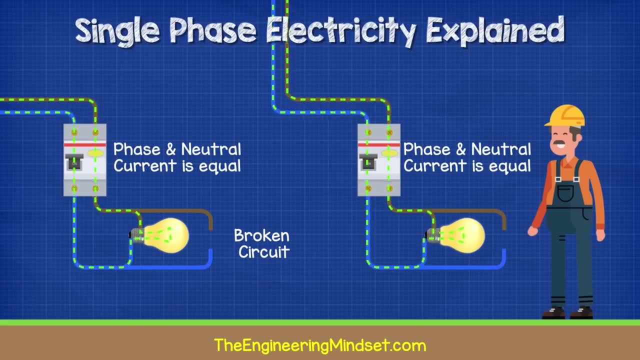 cut the power to everything past the switch. Typically, an RCD will break the circuit if it measures a difference of 30 milliamps, as anything above this is dangerous for humans. If you touch a live wire and electricity flows through you to the ground, 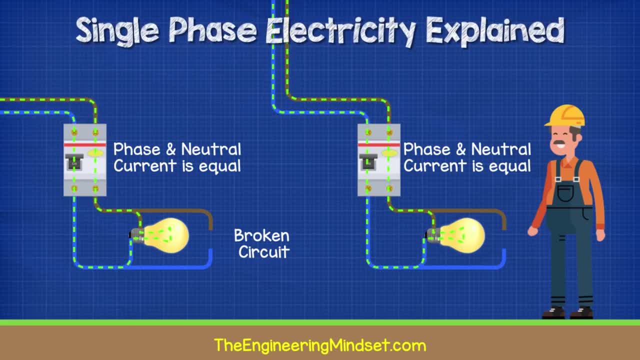 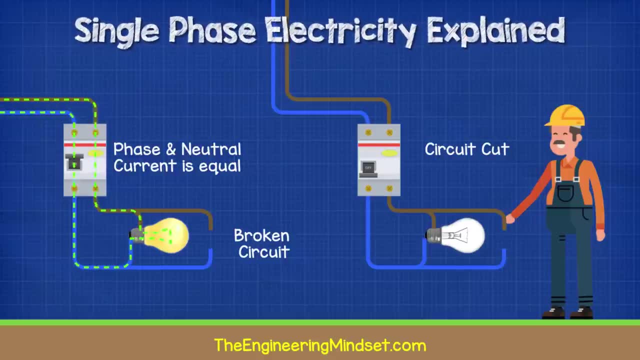 then the current is bypassing the neutral wire, so the phase and the neutral currents will not be equal. The RCD will notice this and then cut the circuit to reduce the risk of electric shock or death. It's now increasingly common to have two or more RCDs. 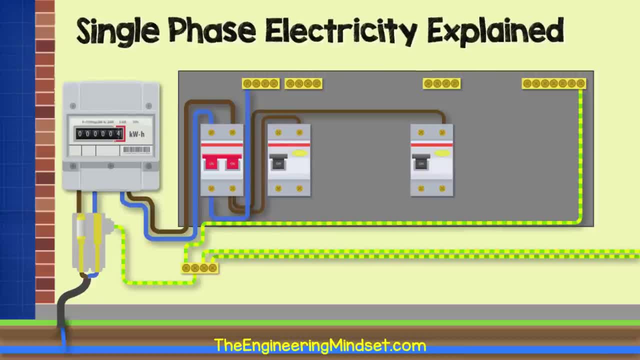 in a consumer unit. In such case, the RCD will only cut the power to the circuits connected directly after it, so the other RCD will still be powered and only some parts of the property will lose power. The RCD will trip when it believes the current is unsafe. 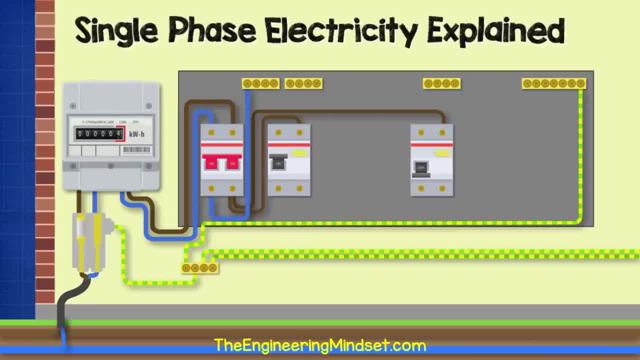 even for a fraction of a second. It does need to be manually reset to restore the power. but this does not solve the problem and you should locate and remove any faulty appliance or fixture From the bottom of the RCD. we have a buzz bar. 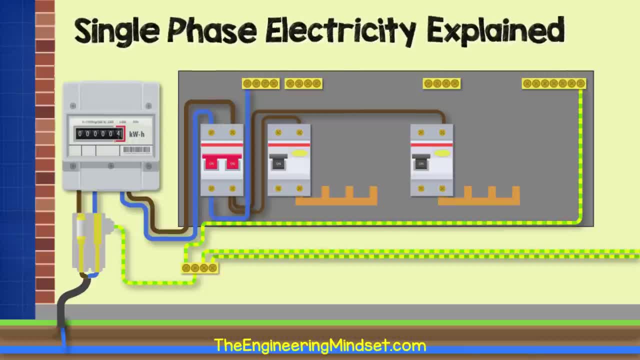 This is just some conductive metal which the electricity flows along and connects into each of the MCBs, which just makes the installation easier rather than having a lot of cables. The RCD, or miniature circuit breaker, controls individual, smaller circuits, For example, connected to one RCD. 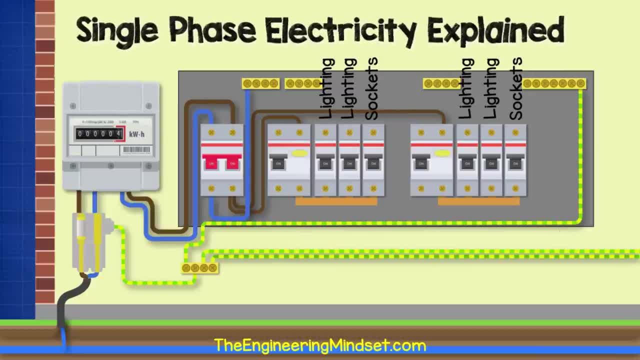 maybe we'll have one MCB for the downstairs lighting, one for the upstairs lighting and one for the kitchen plug sockets. On the other, RCD, maybe we have one for the stairwell lighting, one for the upstairs lighting and one for the downstairs plug sockets. 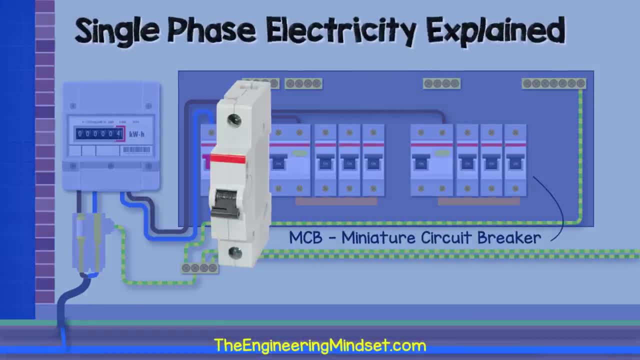 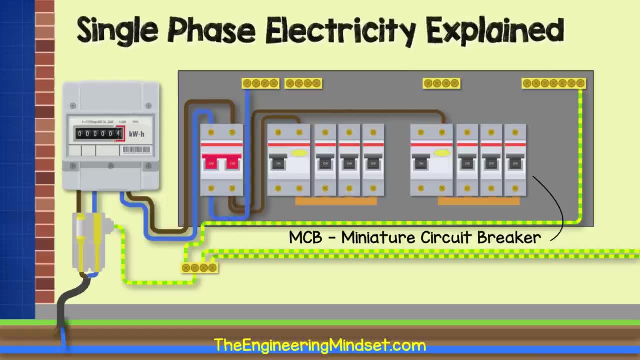 These switches will quickly and automatically trip to cut the power, but they also need to be manually reset to restore the power. The MCB protects the circuit from overload and short circuit. The MCB is rated to handle a certain amount of current passing through it. 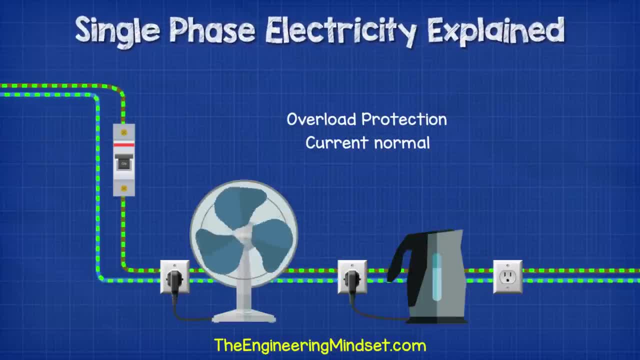 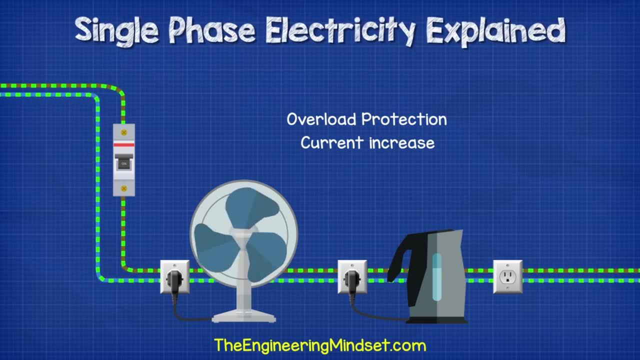 for example, 32 amps for the plug sockets. If this value is exceeded on that circuit, for example by gradually plugging in too many things, then the MCB will trip and cut the power to protect itself. The other protection it offers is short circuit protection. 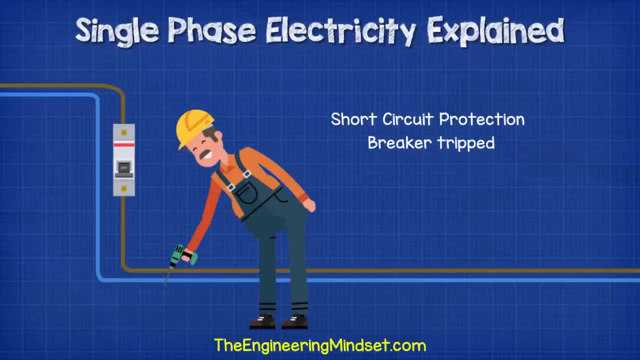 In the event of a short circuit, for example, the live touch is the neutral. then the circuit is bypassed and there may be a large and instantaneous increase in current. This will create a magnetic field inside the MCB which will cut the power to protect itself. 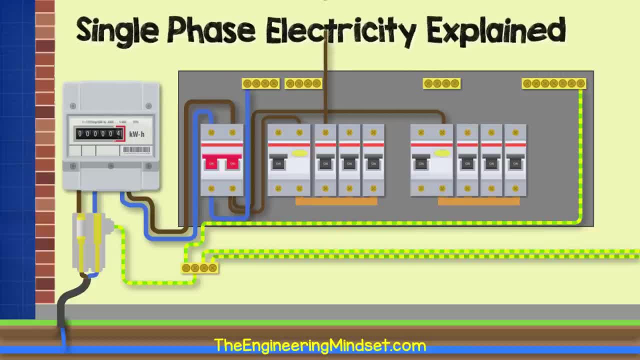 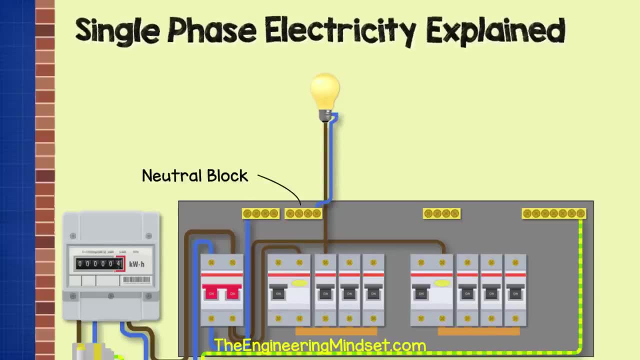 The phase then leaves via the top of the MCB and will flow through the circuit, for example through some lamps. It then returns via the neutral cable and into the neutral block. All the circuits do this, with the phase coming out of the circuit breaker and heading off around the property. 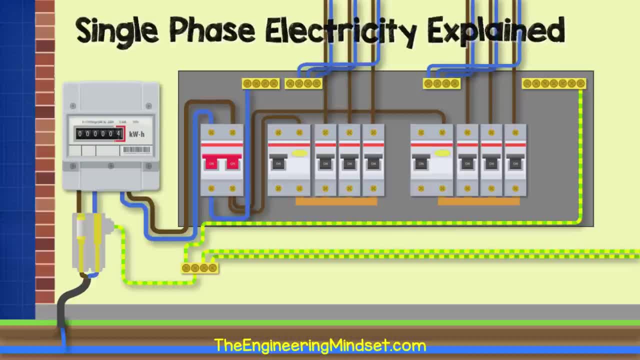 and the neutral lines coming back and meeting at the neutral block. The neutral block is then connected to the RCD, which checks if the current flowing in is equal to the current flowing out. The neutral then flows from the RCD to the main neutral block. 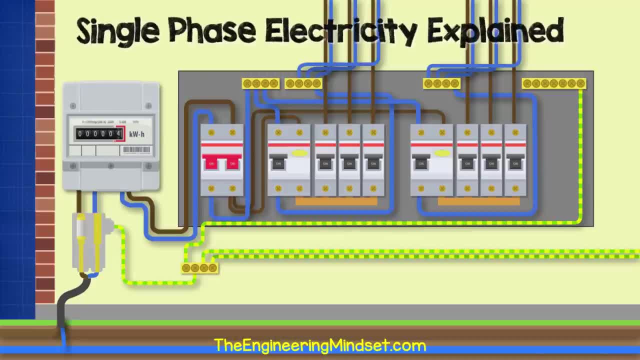 and from there back to the main switch, which is connected to the electricity meter and the service head. So electricity can then flow from the main distribution phase line up through the service head and the main fuse. It then flows through the electricity meter and into the consumer unit main switch. 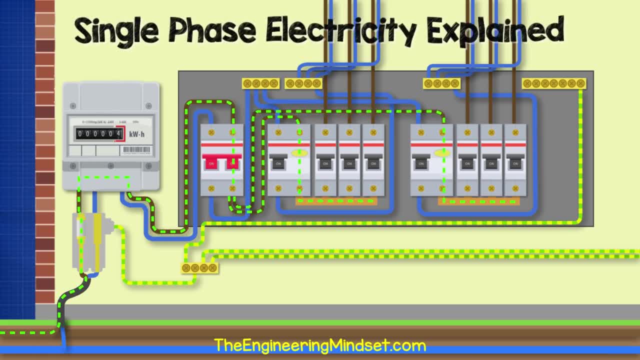 From the main switch. it flows through the RCD along the bus bar and into the MCB. It then flows up around the MCB separated circuit. The electricity can then come back via the neutral lines and into the neutral blocks. It then flows through the RCD and back into the main block. 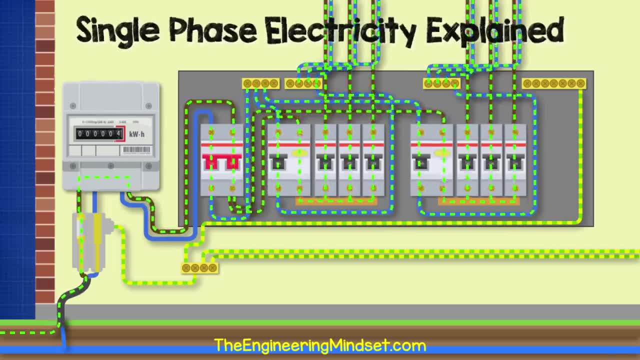 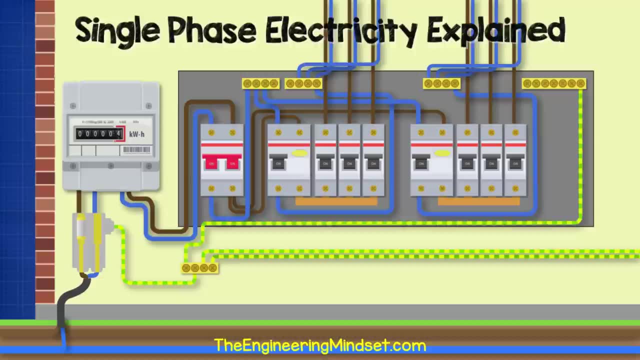 From there back into the main switch and then the electricity meter. It will then pass through the service head and the fuse and back into the neutral line of the main distribution cables. Now you may have noticed that there's some other cables with green and yellow stripes.